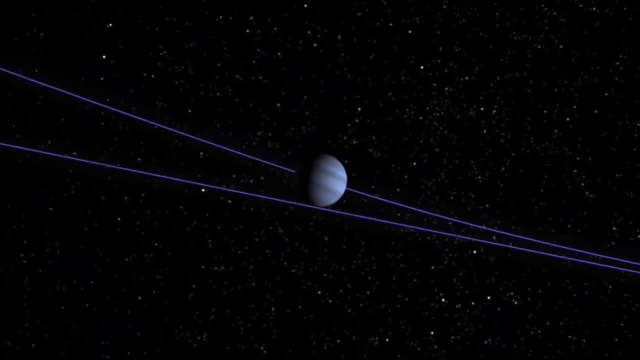 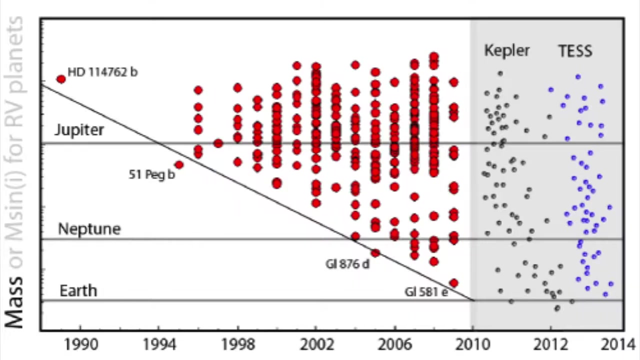 only created for the moon and Jupiter. In fact, there are also many other planets on the solar system. A plot of the discovery of planets in these last 20 years around other stars gives a sense of the dramatic progress. This is a logarithmic scale of mass and the limit on mass detection for planets has marched. 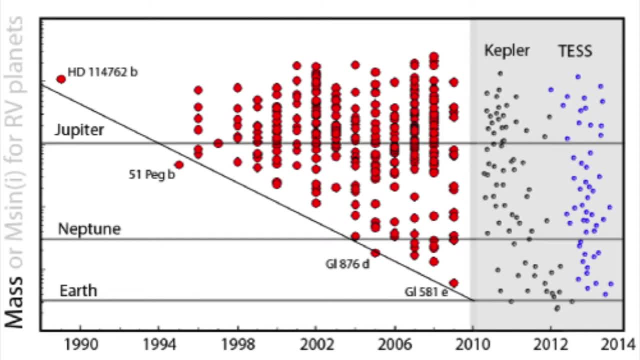 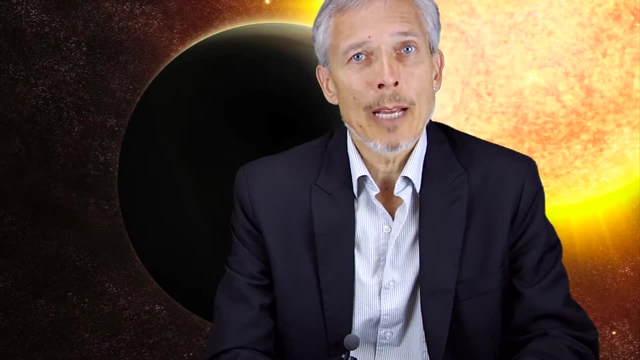 steadily downward from the initial discoveries, which were Jupiter mass or larger, to reach Earth mass just in the last few years. The last couple of years has been overwhelmed by the discoveries from the Kepler telescope in space launched by NASA, In addition to the steady march of a downward mass limit on the lowest mass planet detected. 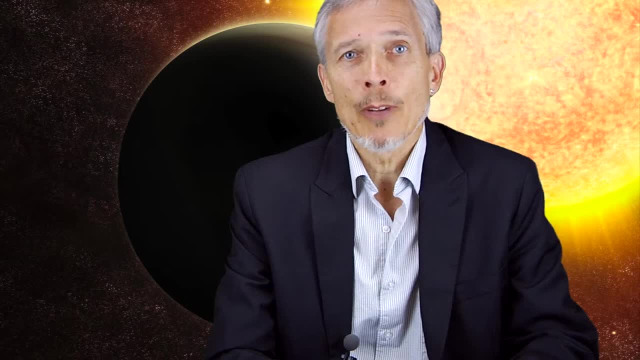 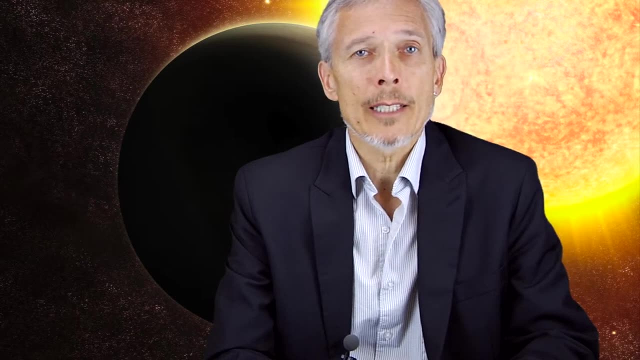 the numbers have continued to accumulate, with a doubling time in the number of exoplanets of between 18 and 24 months. Extrasolar planets, or exoplanets, are one of the most hot topics in astronomy at the moment. The first discoveries puzzled astronomers enormously. 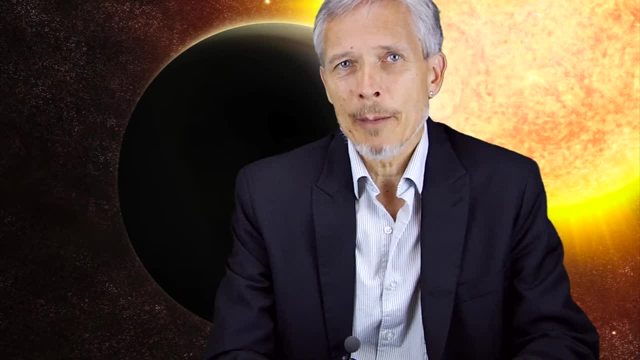 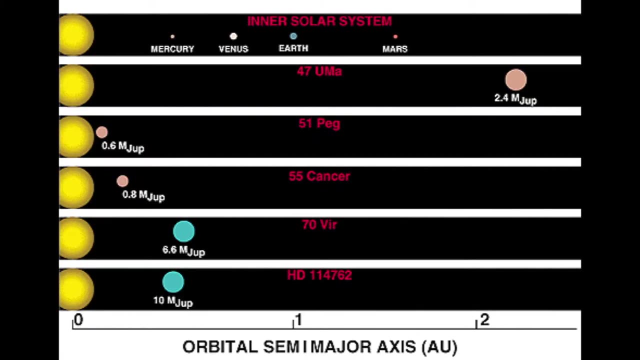 Because, rather than finding giant planets in typical giant-planet orbits, they found hot Jupiters on incredibly tight, hot orbits of their parent sun-like stars. Their very first exoplanet discovered, 51 Peg, is in a 4.4-day orbit around its sun-like star Think. Mercury takes 88 days to orbit the Sun. So this is a Jupiter mass planet far closer to its star than Mercury is to the Sun. Many of the early discoveries were like this, And astrophysicists were confused because they had no way of explaining how giant planets 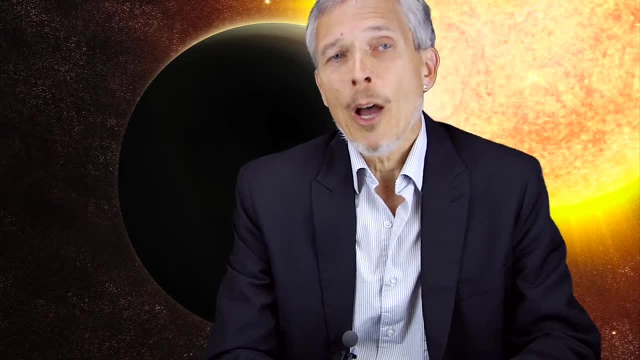 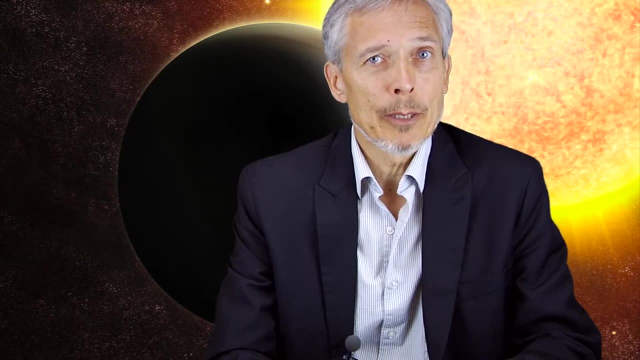 could possibly form so close to their parent stars. Even with a hundred or so detections coming in in the late 1990s, it was clear that there were lower mass planets ready to be found. The distribution of masses of the planets found at any point in the last few decades. 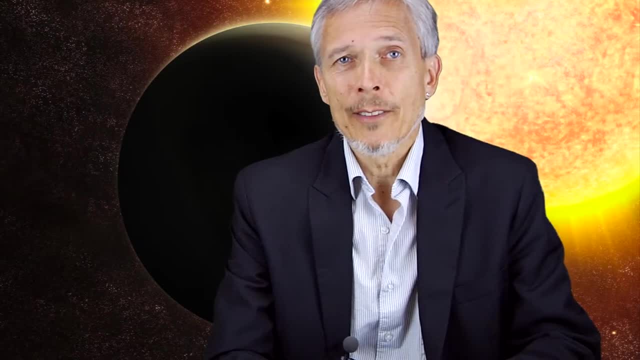 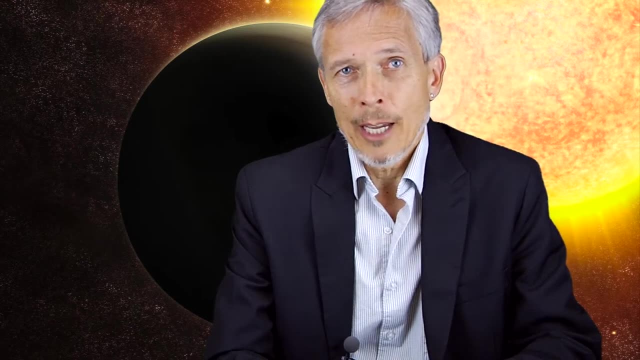 rises rapidly towards the detection limit, That's always a sign that there are low mass planets lurking just below the detection limit. Imagine you are a fisherman, You have a net with one-inch holes And your net was filled with fish. maybe a few that were a few feet long, many that were. 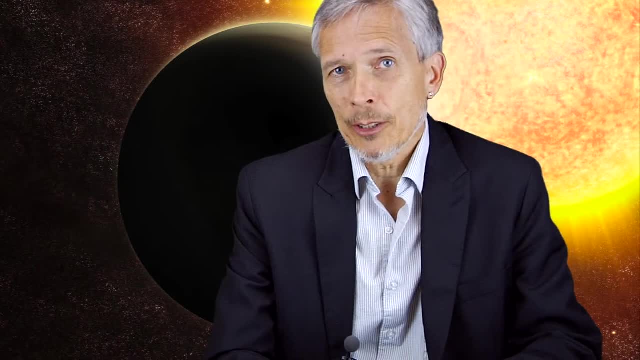 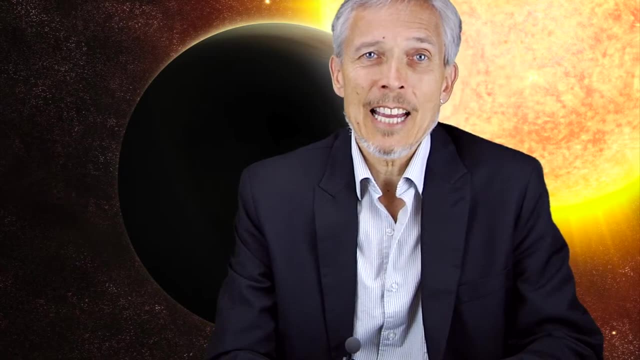 a foot long and a large number of three or four inches bigger than the whole size of your net. The rising number of fish towards the size of holes in your net is an indication that there are indeed many fish to be found that are just too small for your net to catch. 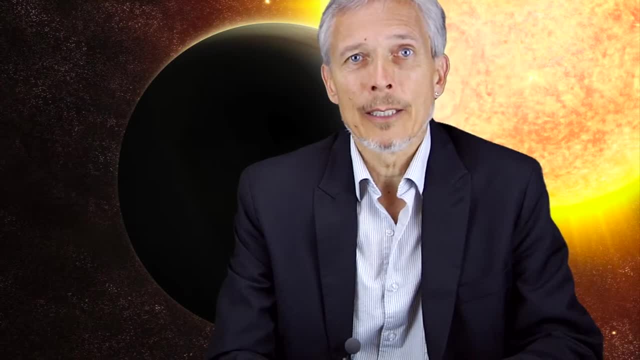 Astronomers also have needed better nets to net the small planets that are out there. As of early 2013,, there were only a handful of fish that were found, And that's why they were so small. There are over 3,000 exoplanets known. 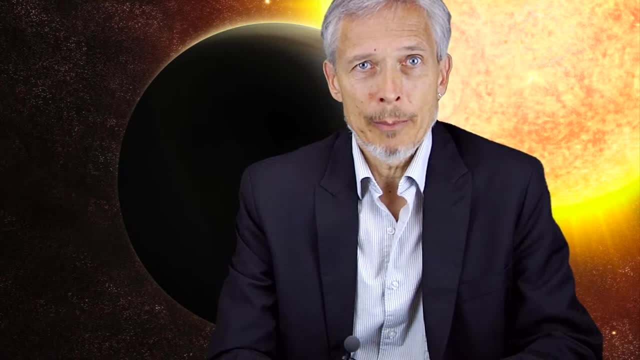 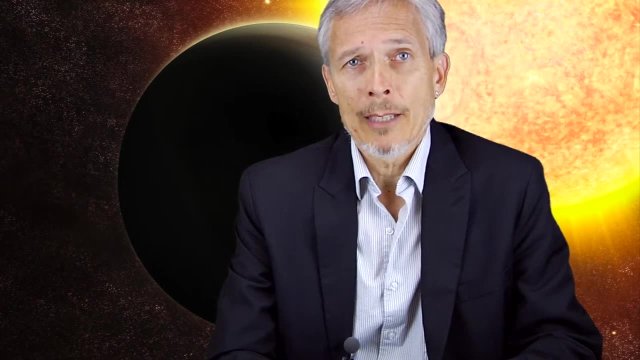 Many of these remain to be confirmed, but in all likelihood they will be, because Kepler detections have a 90% probability of being confirmed once they have sufficient data. Many of these are Jupiter mass and most are more massive than Uranus and Neptune. 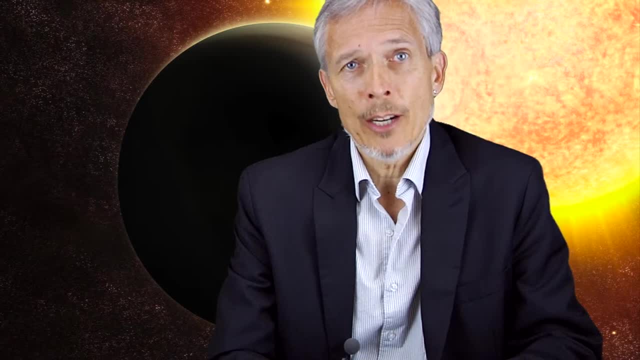 But gradually, the detection limit has reached towards super-Earths and Earths, And there's every expectation that a very large number, perhaps the majority of exoplanets are small, rocky terrestrial planets. The presence of so many giant planets so close to their stars forces a revision of our idea. 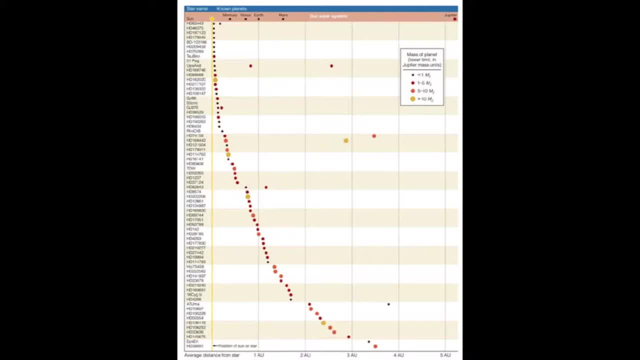 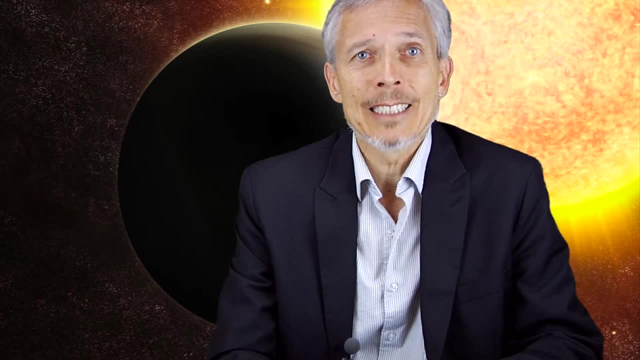 of how the solar system formed and other solar systems, Because there's no way for planets to form that large, that close, There's not enough material and there's no way for that material to condense and go into an object in a stable orbit. 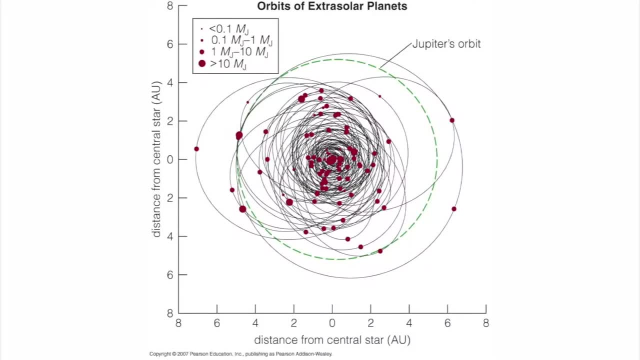 The early exoplanet discoveries had other puzzles too. When people plotted out the eccentricity of the orbits or the degree with which they deviate from circularity, these planets were in much more elliptical or more elliptical or more eccentric orbits than the planets in the solar system. 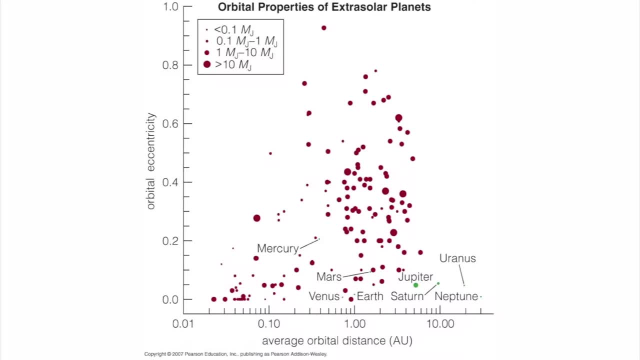 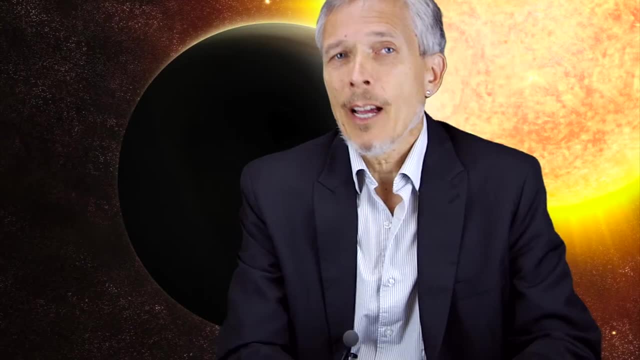 In fact, most of the first few hundred exoplanets had eccentricities of 10 or 20%, which is rare in the solar system. Nobody could explain why the orbits were so eccentric. The excitement of discovering exoplanets was tinged with frustration, because people could 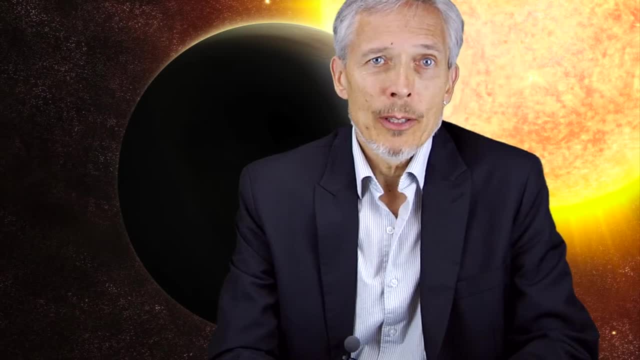 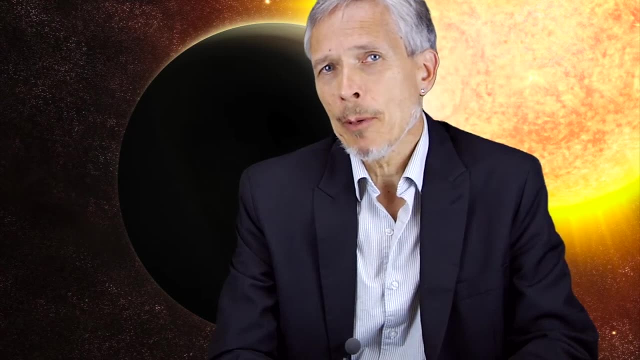 not explain how these planets formed. It seems now that planets can migrate and that planetary migration has to be a standard part of the way solar systems work. Not only that, Planets go through periods in the history of a solar system where their orbits are unstable. 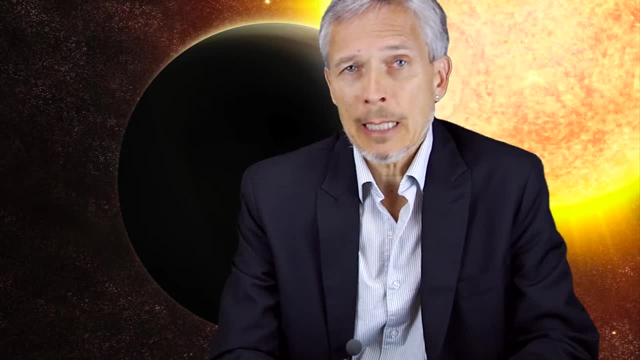 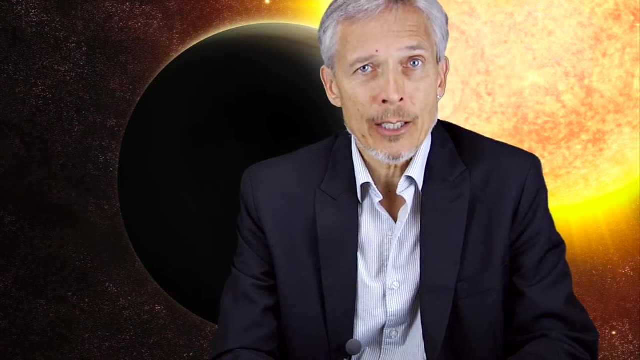 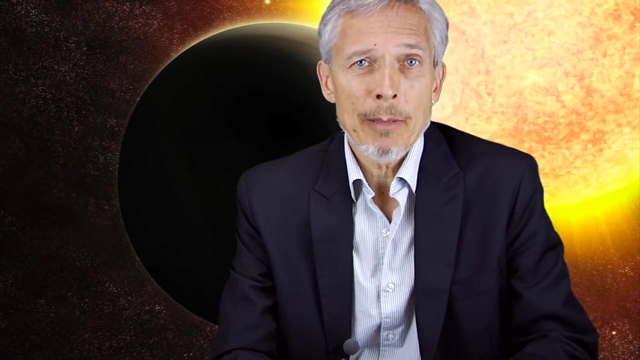 They can change places, move inward or even outward, and occasionally get ejected from the system entirely. Computer models have been essential in helping us understand the chaotic motions and orbits of solar systems. These new models applied to our solar system suggest that the giant planets have not always 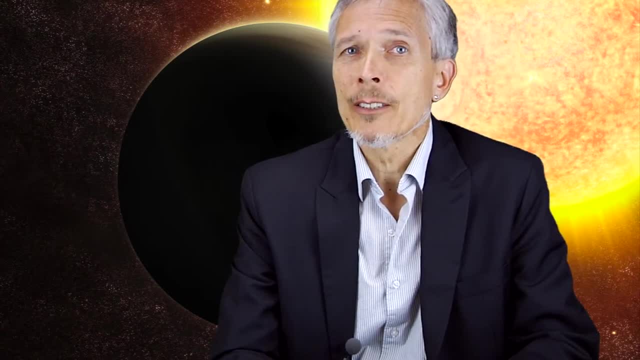 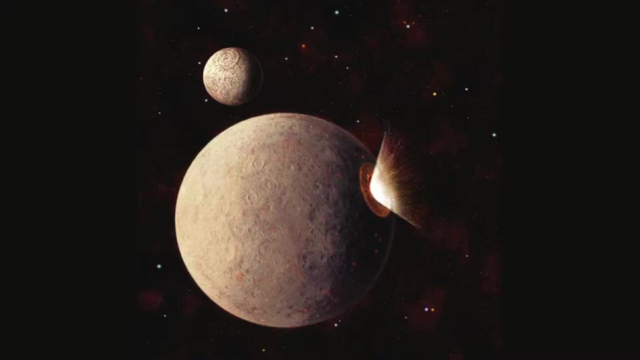 been in the positions they hold now. In fact, there's indirect evidence that Uranus and Neptune swapped places early in the history of the solar system and that this rearrangement was associated with a perturbation to the comet cloud that produced a spike in the impacts on the Earth and the terrestrial planets. 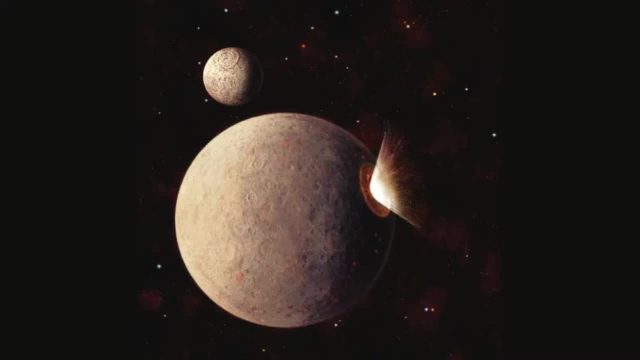 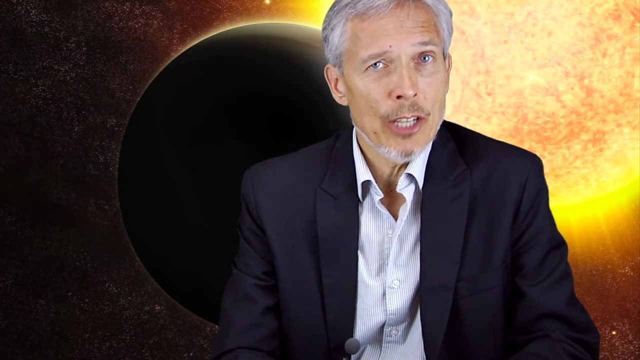 If true, this solves a mystery of several decades standing whereby there's an era of heavy bombardment about 3.8 to 3.9 billion years ago, present in the cratering record on the Moon and Mars and Mercury. There needs to be a reason to explain this heavy bombardment because, in general, after 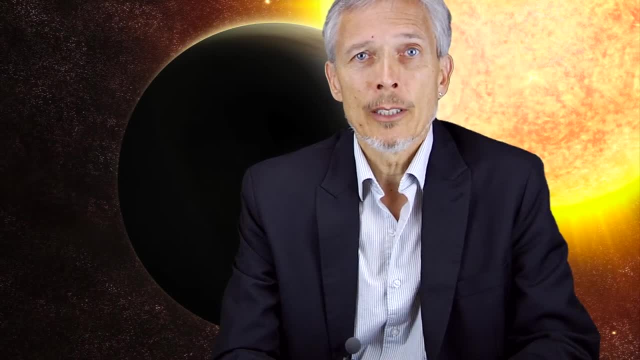 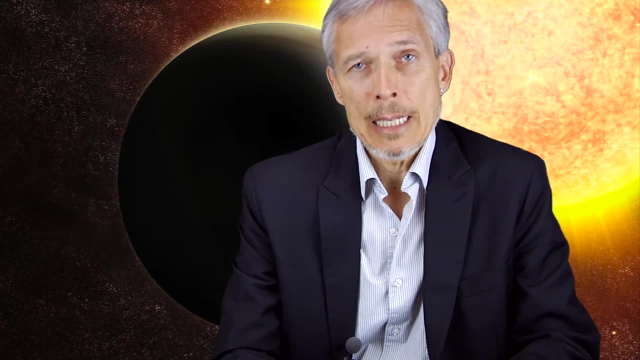 a solar system formed. the amount of heavy rocky debris objects diminishes with time as they form planets and are swept away. There should be a continuous decrease in the cratering rate. Instead, we see a spike- 3.8 to 3.9 billion years ago, presumably impacting the Earth. 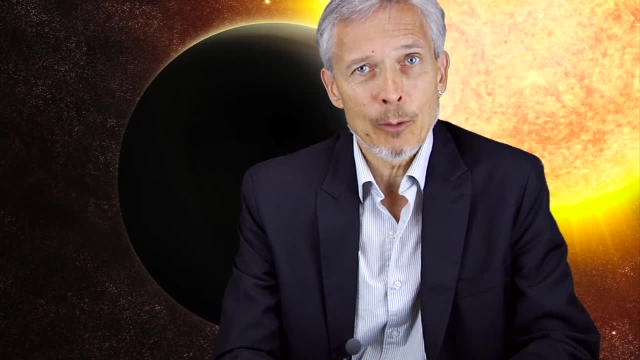 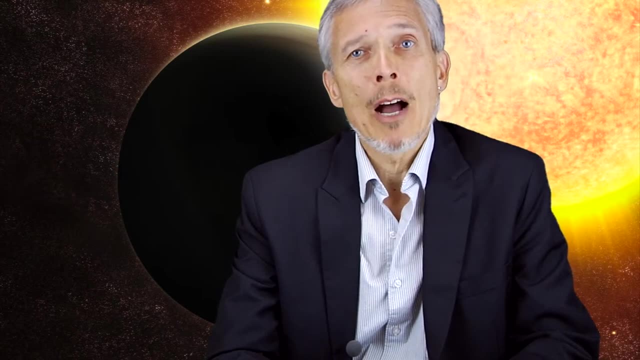 too, but the cratering record is not good on this planet because of erosion and tectonic activity. In some ways we can think of the way planets behave as a game of cosmic billiards. a very violent history early on as the planets formed. And then occasional violence later on as the planetary systems go through instabilities. Some of these instabilities are triggered by resonances, such as when giant planets enter orbital states where the ratio of their periods is a whole number 2 to 1, or 3 to 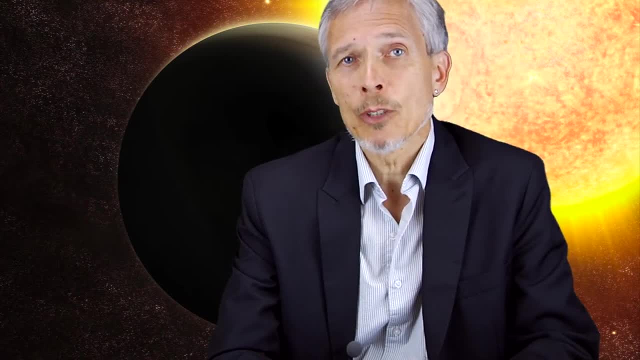 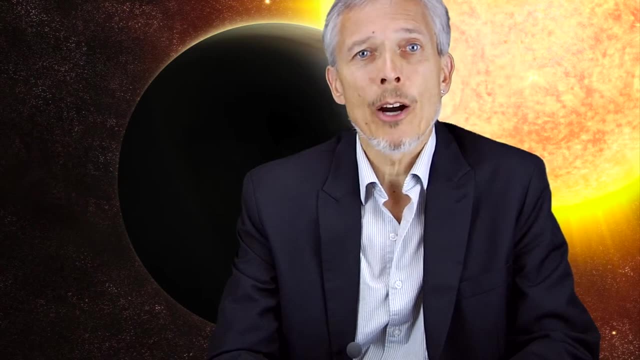 1, or 3 to 2.. These resonances have been observed in the moons of giant planet systems, but they could apply to the giant planets themselves. Planetary migration is now a standard part of the theory of how solar systems form. Put simply, it is impossible to form a high-level solar system. It is impossible to form a high-level solar system. It is impossible to form a hot Jupiter in its place. It must have formed further out and migrated in. While migrating in, it might fall into the parent star or park in an orbit and form a 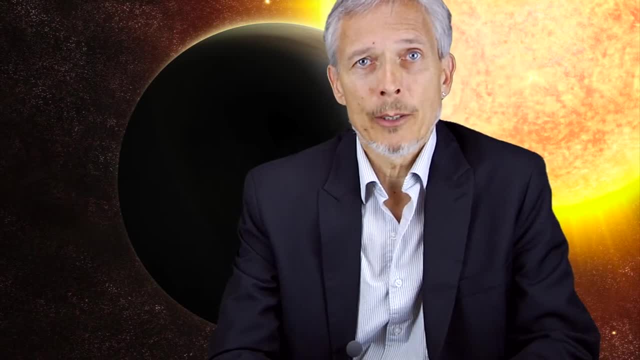 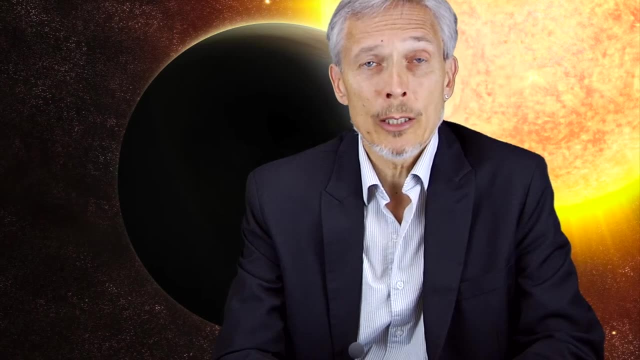 stabilized facing position, tidally locked to the parent star. No one was present when these events happened, so it's very hard to verify these models. We have to look for subtle clues in the current placement of the planets and in the behavior of the comets, asteroids and meteors. Another way to think of this is the fact that the solar system is essentially full. In dynamical terms, we can visualize the solar system, and we know that the space between planets is vastly larger than the size of the planets themselves. The solar system, indeed, seems like mostly empty space. 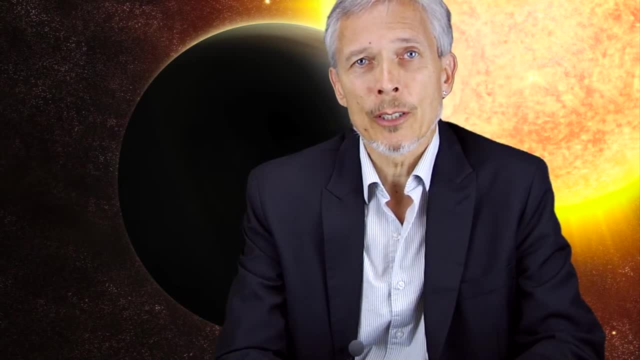 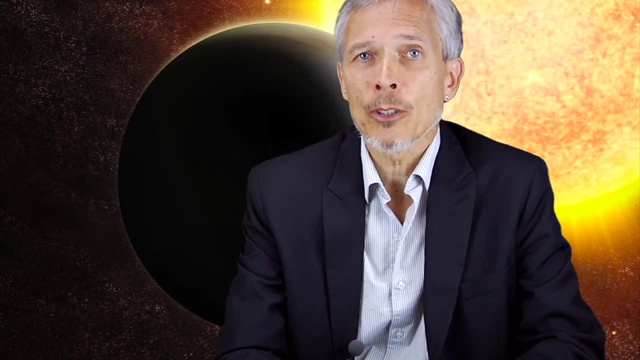 But if you play a game in a computer where you take the current arrangement of the solar system and try to drop a small terrestrial planet somewhere else, such as between the orbits of Mars and Venus or even in the outer solar system, it causes chaos. 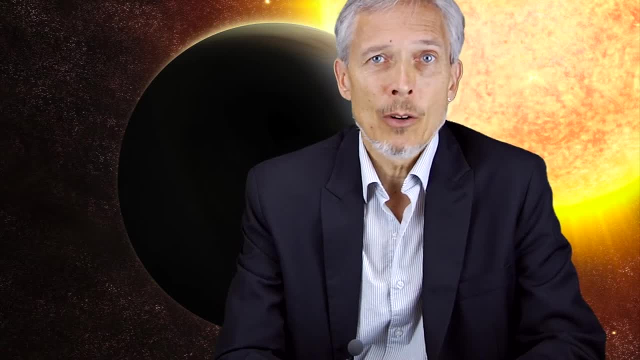 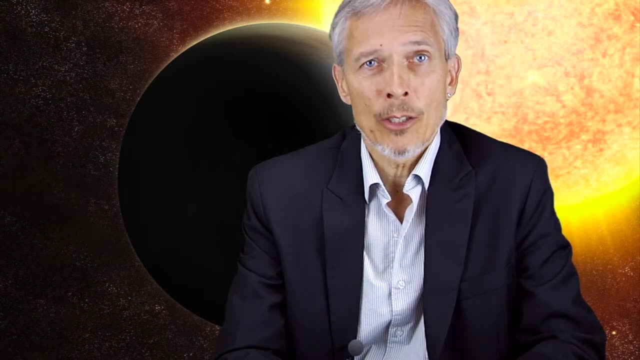 It upsets the orbits of the giant planets and occasionally ejects one from the system. In that sense, the solar system is full. It contains about as many objects as it could and still be long-term stable. The solar system, having undergone rearrangements early in its history, does now appear to be 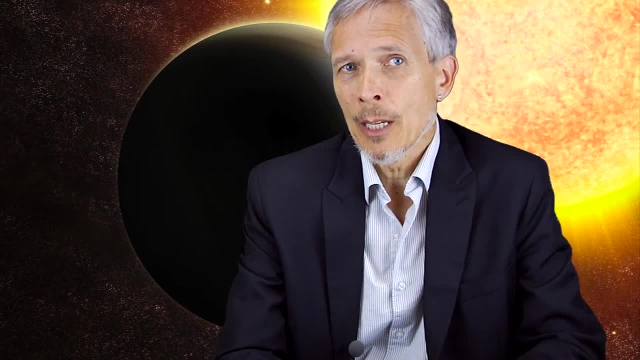 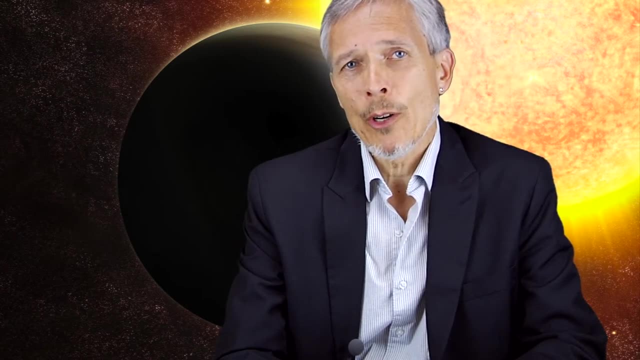 stable. If we run these models forward for our solar system, the planets stay in their current orbits for at least a billion years. The models with good computers are now capable of showing how terrestrial and giant planets might have formed. We have plausible creation scenarios. 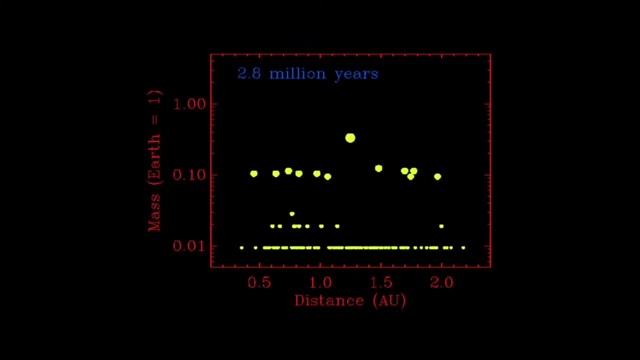 For terrestrial planets, it's essential to know that they're not just planets, they're planets. This is a situation where planetesimals, rocks of maybe a hundred to a thousand kilometers in size, about the size of the largest asteroids, maybe a few thousand- are present. at the beginning, 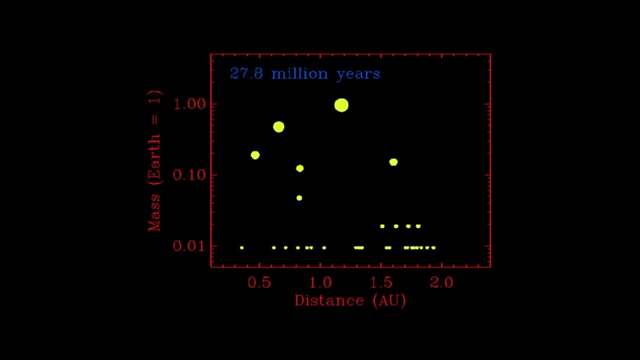 and in a few tens of millions of years they collide, accrete and form a set of rocky planets. Running these simulations over and over shows the possible arrangements of terrestrial planets. in solar systems like ours, The process takes place relatively quickly, occurring within tens of millions of years. 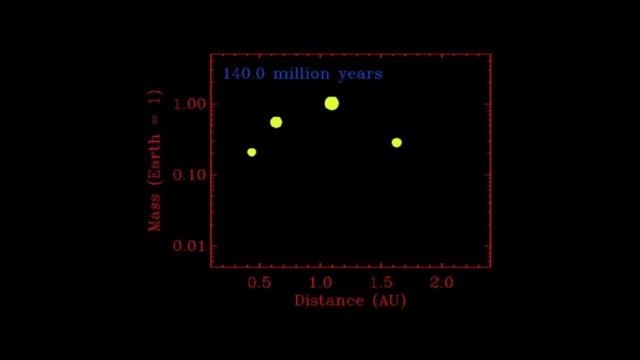 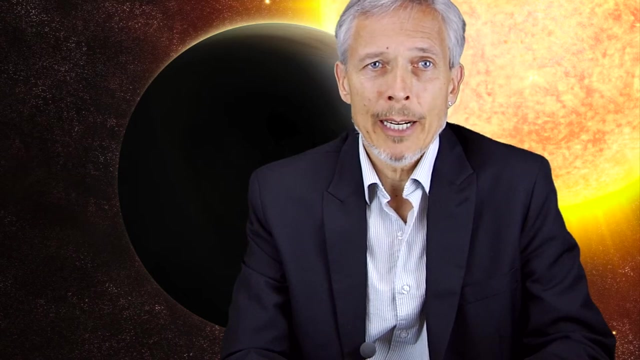 after formation. This is a tenth of a percent of the age of the solar system. Gas giant planets form in an analogous way. There are rocky cores to the giant planets that form by accretion And then, because there's much more material at the periphery of a solar system, they accrete. 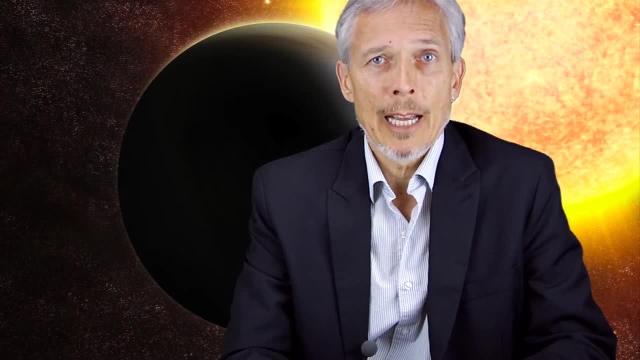 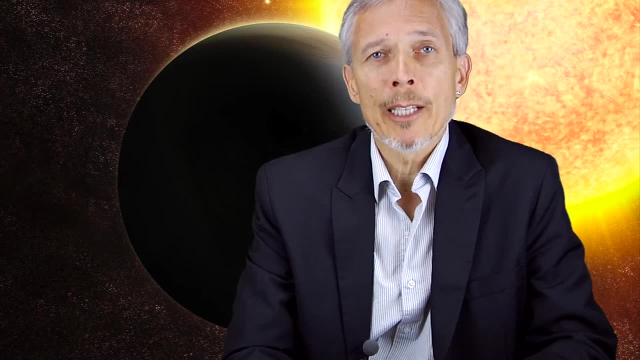 hydrogen and helium mantles and so become large gaseous planets with the same chemical composition as the sun. Those planets sometimes migrate rapidly inward, sometimes falling into the parent star, sometimes parking in orbits where we might detect them as hot geysers. 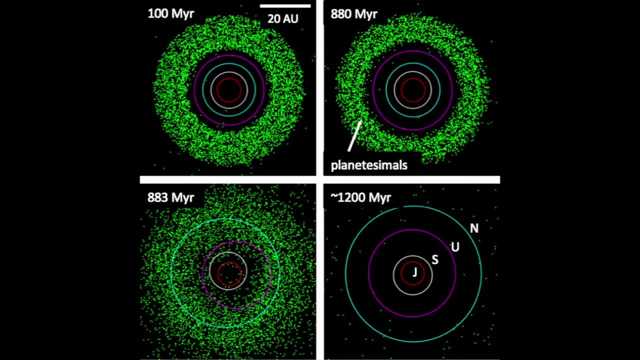 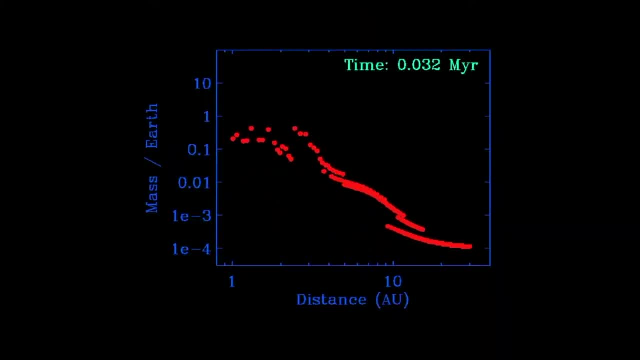 The stable Jupiters and Saturns take longer to form and they stay further out tens of astronomical units from their parent stars. Simulations show how this might happen and confirm that migration and parking of a giant planet is something that we should expect to happen. 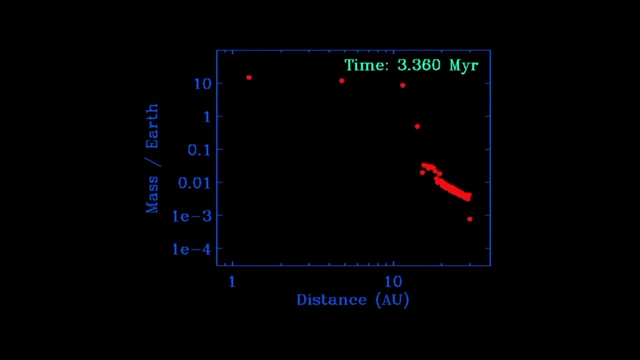 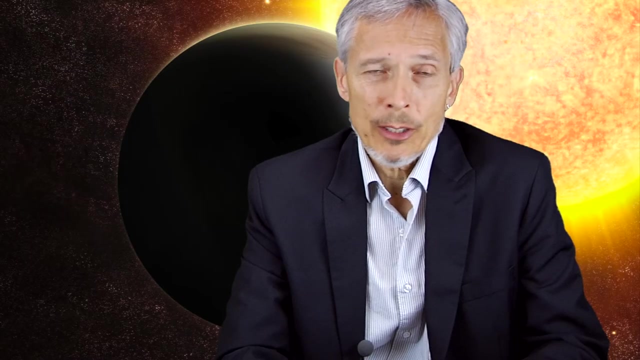 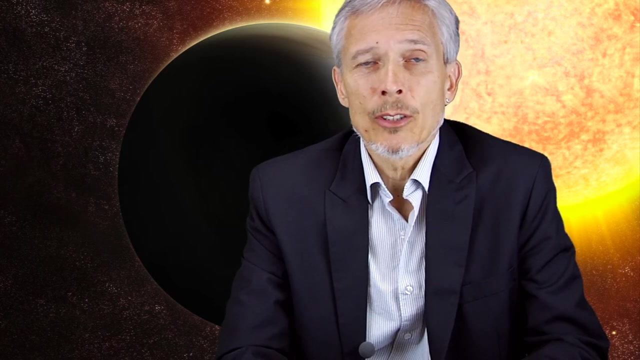 What might planets around other stars look like? What might other solar systems look like? Before the discovery of these solar systems, we had no idea, But it turns out that nature is quite imaginative. We can imagine solar systems that might look somewhat like ours or vastly different. 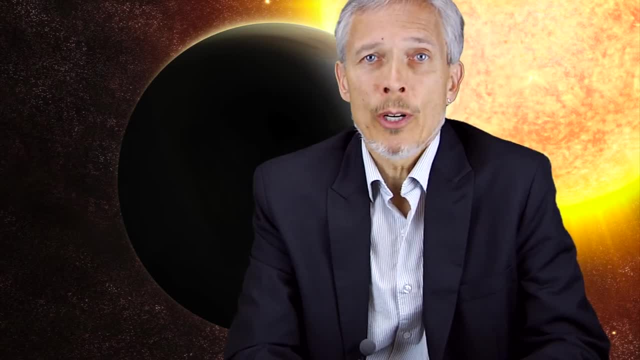 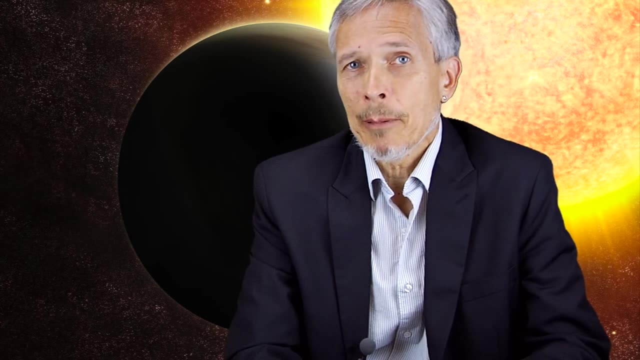 In simulations We can imagine that anything from one to half a dozen or more terrestrial planets are formed, and they're not all the same mass as the Earth. Venus, Mars and Mercury. Equally giant planets can form in diverse ways and in diverse numbers.